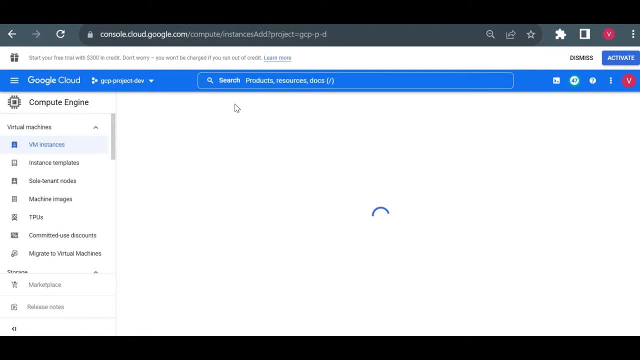 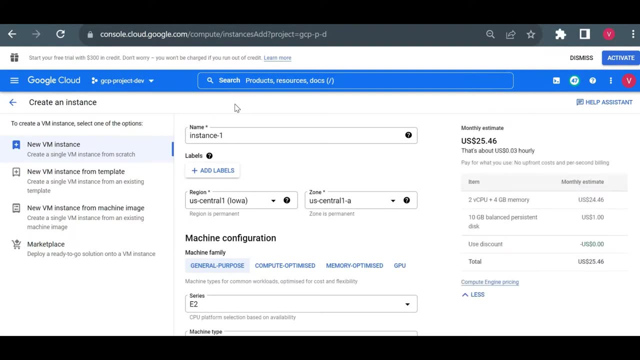 of when you go to buy your own laptop. so what all things you will check for buying laptop? you will just check for ram, you will check for operating system, you check for cpu. so the same specification we have to provide while creating a virtual machine. so here suppose, 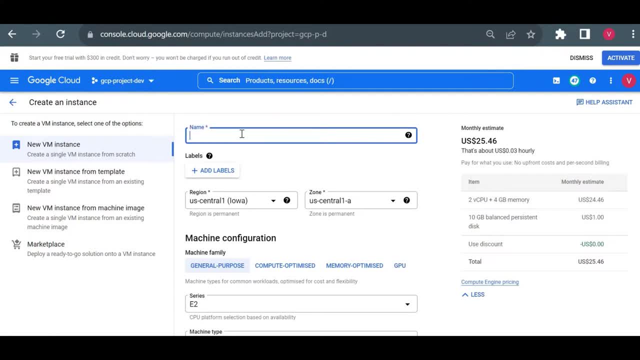 i have to create. i'll just give the name, so name. i'll just give you a demo now: the region and zone. so while you are creating a cloud resources- any cloud resources- you have to specify the zone and region. so we already seen what is regions and zone in our previous video so you can choose a nearest location. 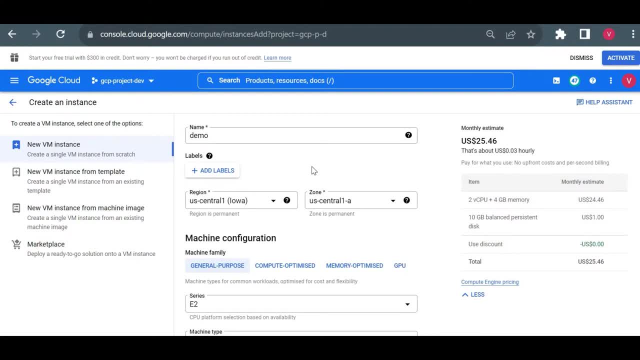 but for this demo i'll just choose us central one because it is the cheaper one. so you could see, your pricing is also based on your regions and zones you are choosing now here you could see: uh, the total is 20 dollar if I am choosing the US and alone. so let me choose South America East one. 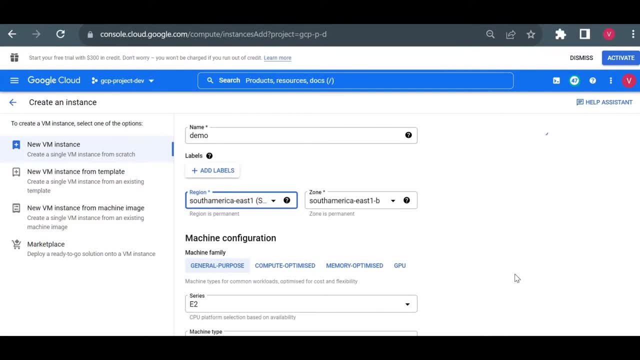 and we'll see the pricing. now pricing is 40, so your pricing will change based on your location, so I'll just choose the lowest. let's use central one, because for this demo this will be cheaper for me and as I was talking about the CPU and 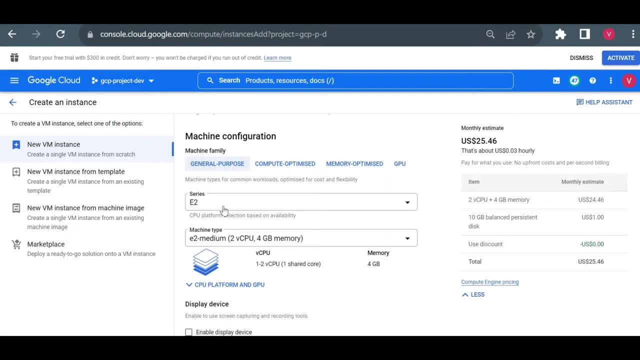 RAM. so it is just, you can configure in machine configuration. so here you just choose a series. so there is a different type of CPU series available. you can check in Google Cloud documentation, so we'll choose the basic one. so here you can choose the C 2 and 2 and 3, so you can find the specification on Google. 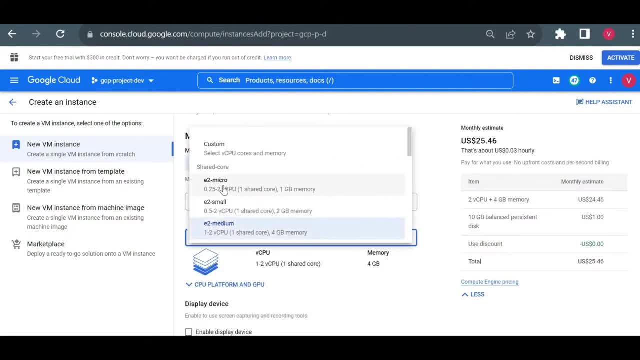 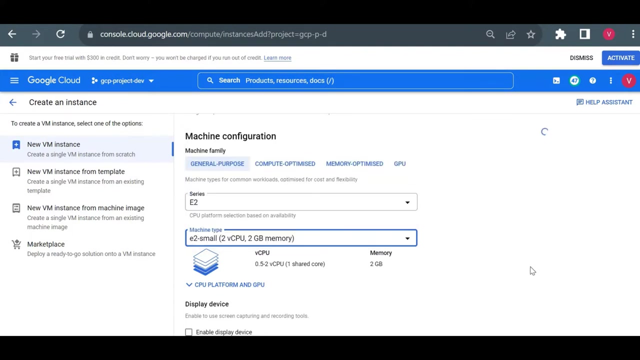 Cloud documentation and I will just choose into micro, which is the smallest one. okay, so it contains two CPU and one GB of memory. so your pricing you could see now reduce to $7. that is for month. now suppose if i go for more i will go for 2 GB. a pricing will increase now the 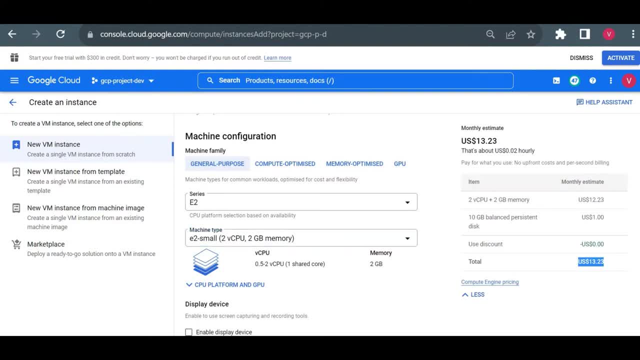 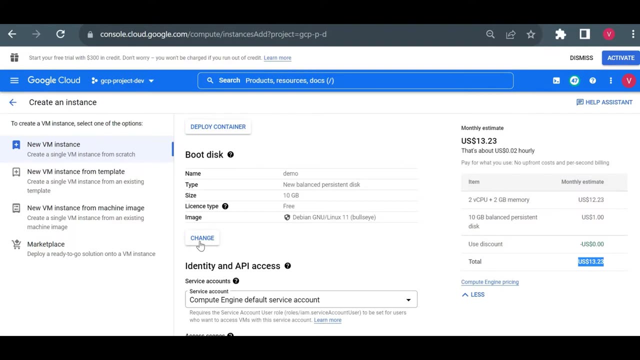 pricing is $13. so the more you, a powerful computer engineer, will choose, more you have to pay for it. now that's read for a machine configuration. now I have to choose a boot D. so what kind of virtual machines operating system I want? if I want a dbn or a Windows or any kind of play, thisんで. 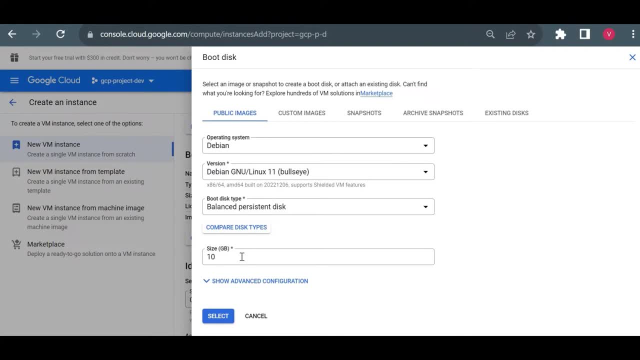 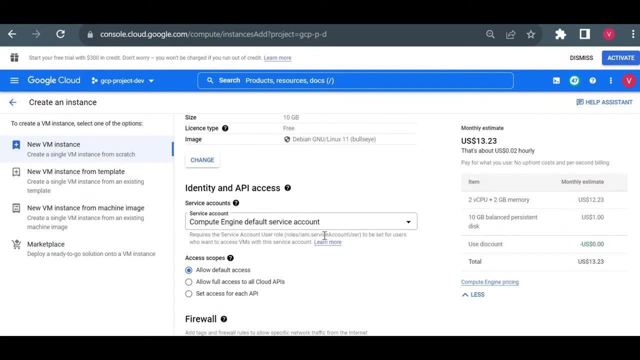 debian one which is default and at the boot this size. i'll keep a 10 gb here so you can specify whatever you want and this service account and all these things. i'm not keep choosing anything customized, i'll keep everything as a default. so here you have option to choose your network. so 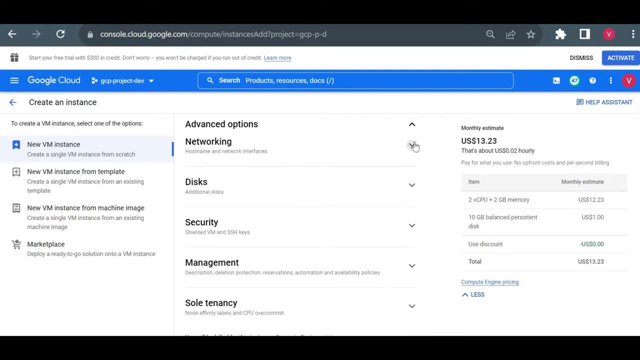 once you start working on vpc you can create your vpc network and create your virtual machine inside your vpc network. but for now it will take a default if you haven't created any network or you haven't specified any network. so here, if you see, i have option to choose a different application. 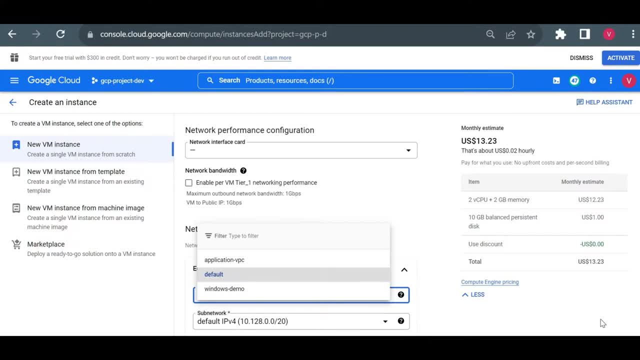 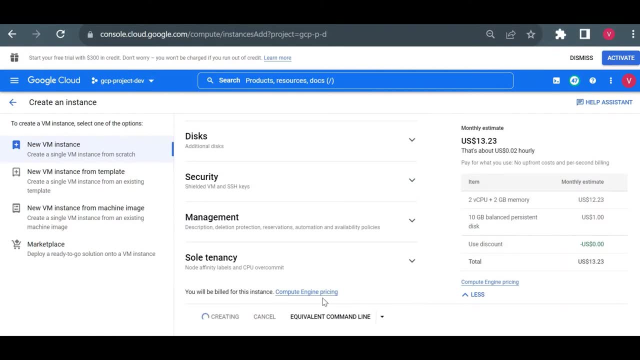 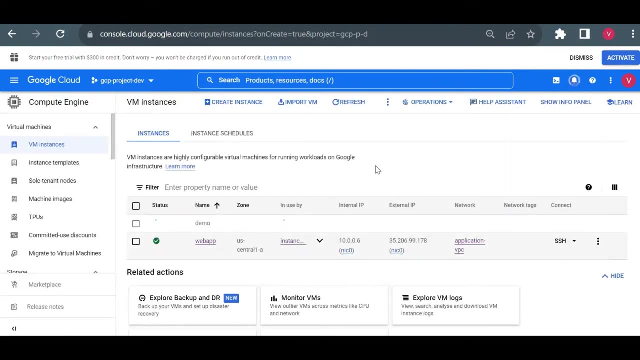 vpc or windows demo network, but i will choose a default network and i'll just go and create. your virtual machine is being created. it will take few seconds to start. your virtual machine instance is up and running. so you could see. the name is demo zone. we specified us central 1c. 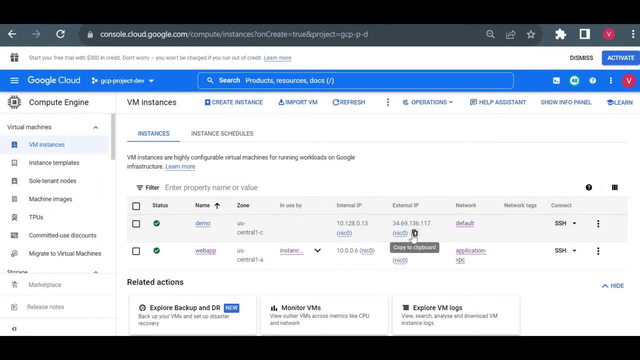 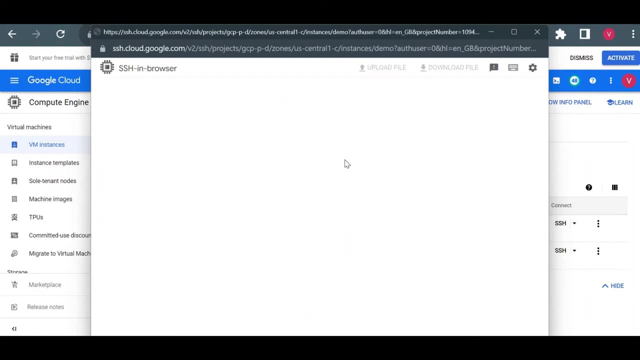 this is your internal ip. this is your external ip, so you'll see in detail about what is internal ip and what is external ip, indeed in another video. and here is option ssh, so you can simply click on this ssh and you can log in into the virtual machine. but for login you should have a firewall in place. 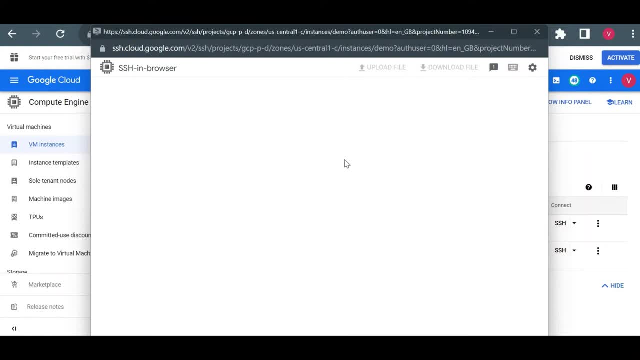 in your vpc so you can see a different video. uh, in my playlist for creating firewalls, creating a virtual private cloud and a subnets. so in this video we are just seeing how we can create a virtual machine in gcp and we are not going in much details on all the parameters. 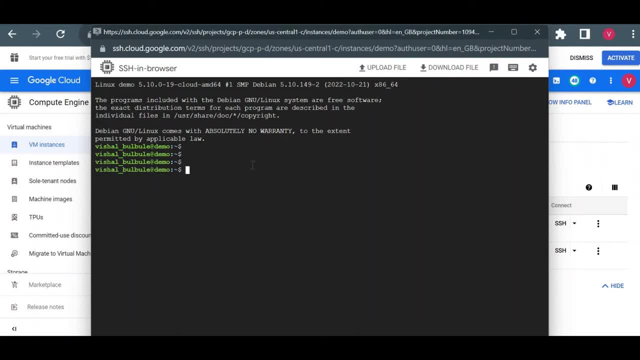 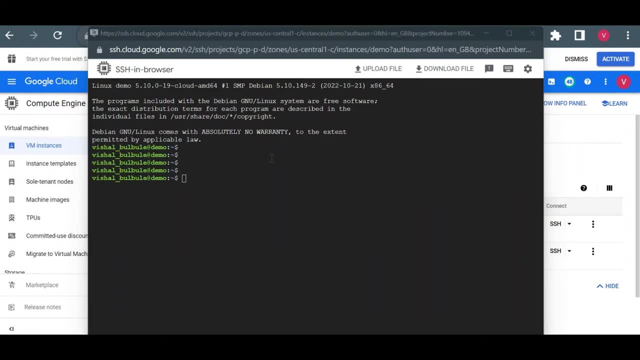 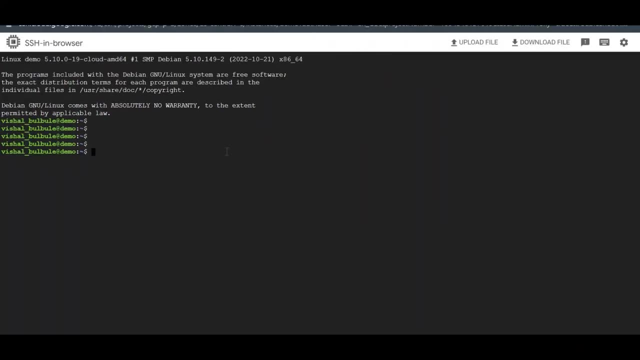 inside your virtual machine. so that's it how we can create a linux virtual machine in gcp now. now you just install a simple apache web server on this virtual machine. i'll just expand this, so we'll just log in as a pseudo first, okay, and now we'll just update the packages. 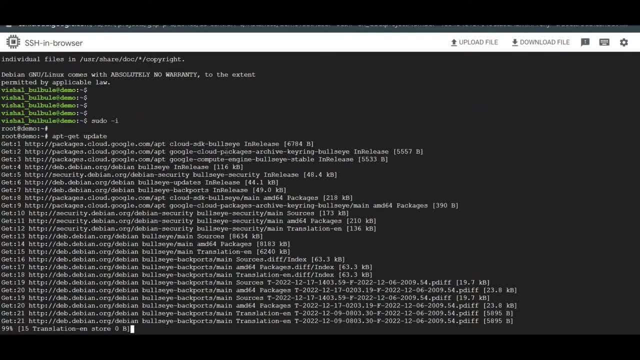 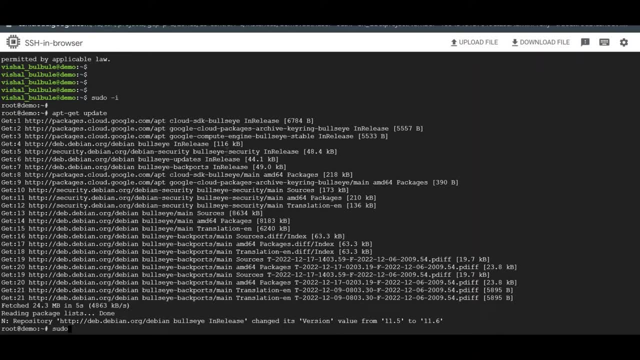 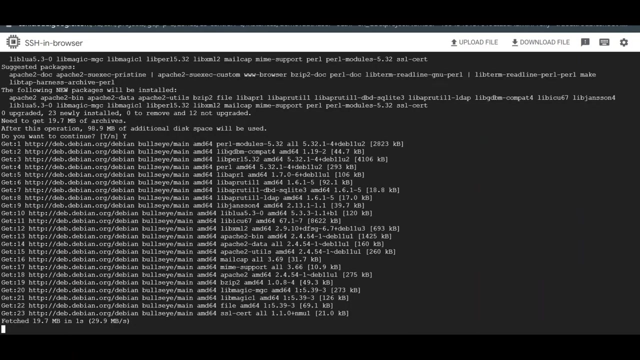 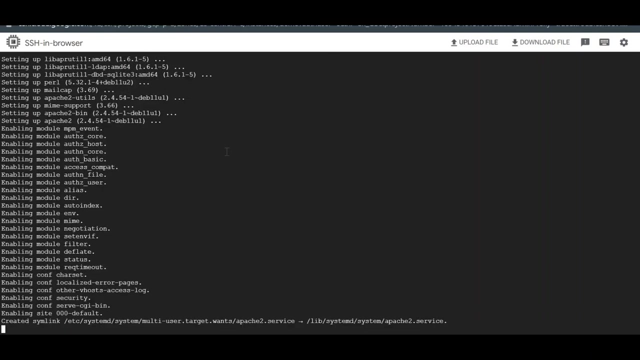 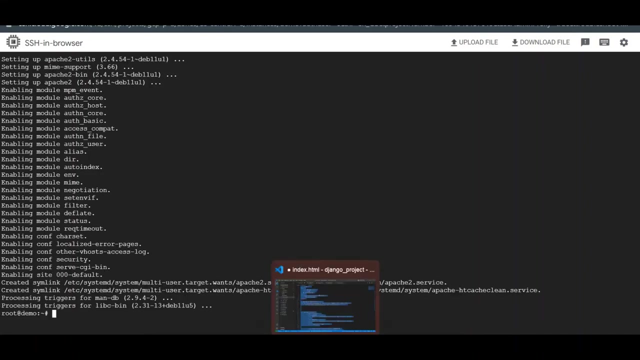 so it will just update the packages in this debian virtual machine and now i just install apache. so so, so, so, so, so, so, okay, apache is installed. now we'll see if it will show anything on the external ip. so i'll just use this external ip and try to check in browser. 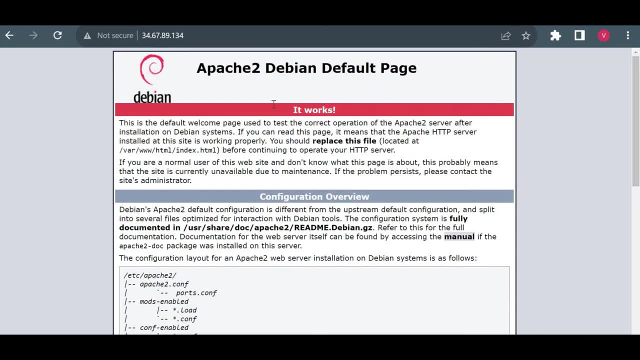 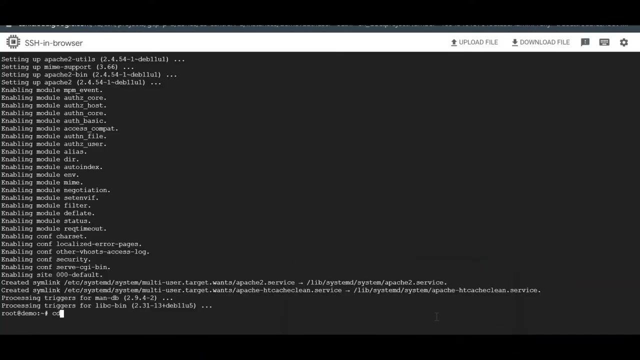 okay, so it is showing this apache debian page because we didn't include it in our html page. so what it is saying: you should replace this file at where- wwwhtml- indexhtml, before continuing to operate http server. so we'll just go to this path and we'll see here. so here we'll have indexhtml. 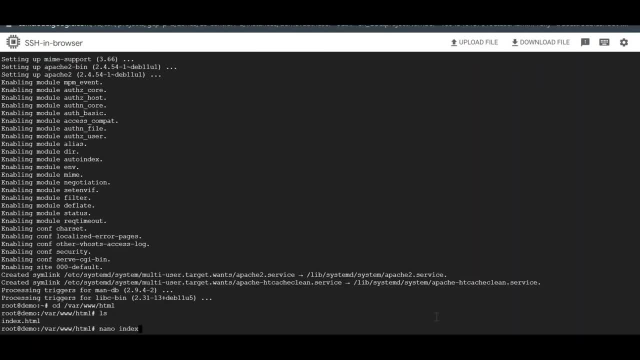 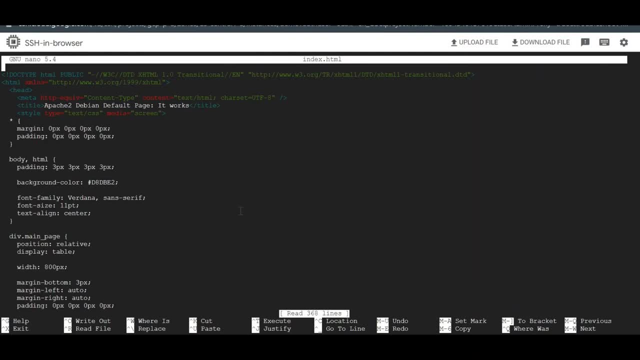 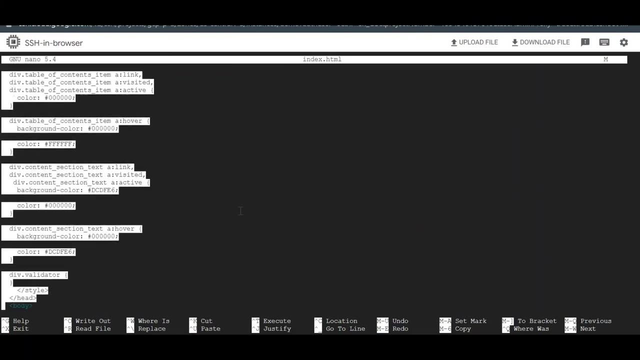 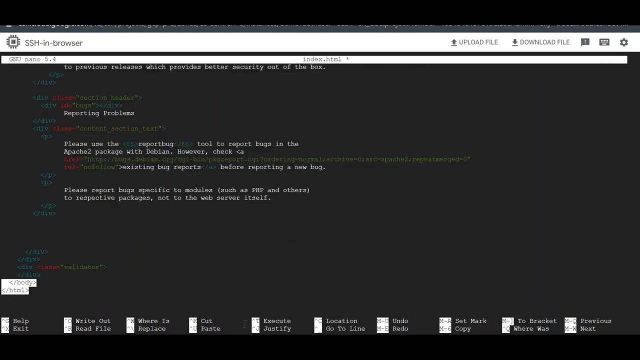 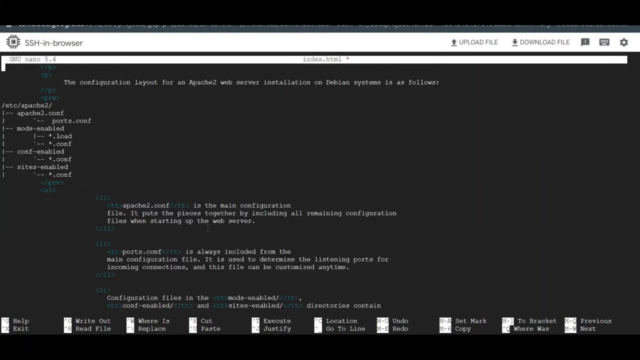 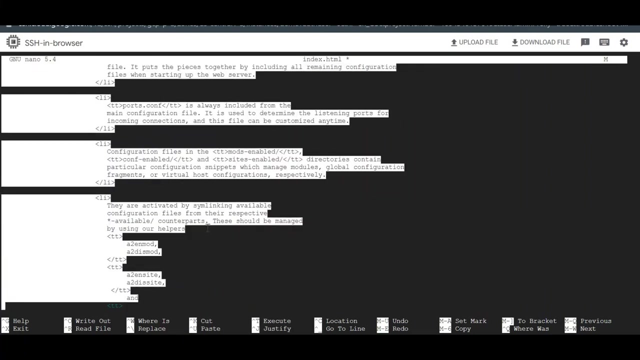 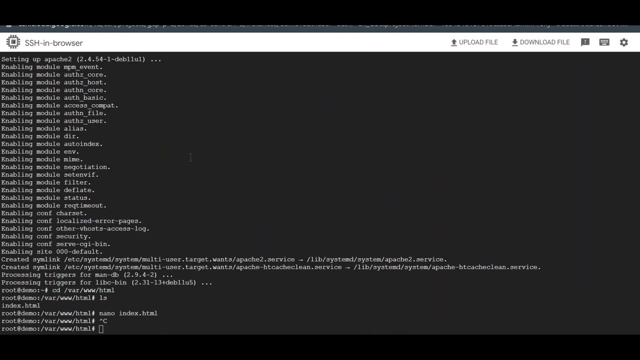 so i'll just update this indexhtml with my code. so i'll just remove whatever is available here and i'll paste my html code in this. okay, i'll remove this. okay, okay, okay, okay, okay, okay. so i'll replace this indexhtml with my html code. so first i'll remove this indexhtml.